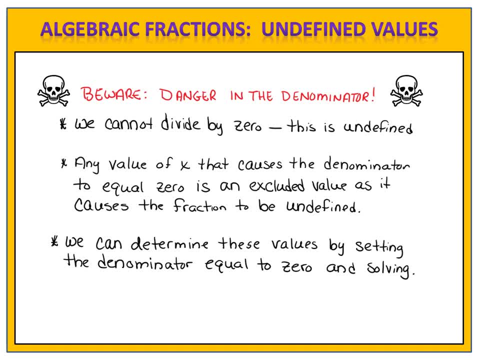 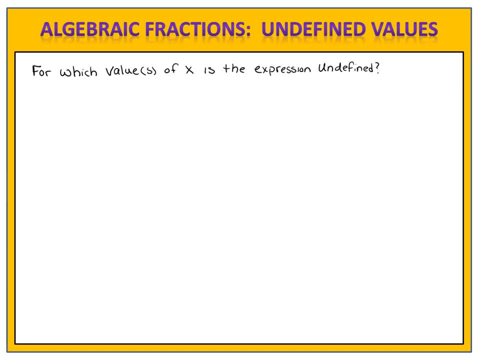 and solving to see the values that cause that denominator to be zero. Let's take a look at a few examples so you can see what I mean. For which value or values of x is the expression undefined? Now, if we divide by 어때, we should conclude that the argument about real divided by zero 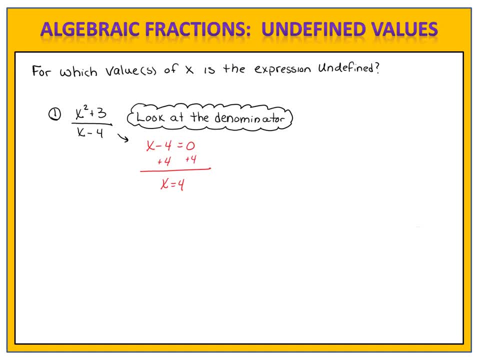 is undefined and that its downside is x square plus c square divided by aıs. Then, tackling this problem from aволence, we are going to give their double чемices definition Here: 4.. This fraction is undefined when x equals 4.. Why is it undefined? Well, make note of. 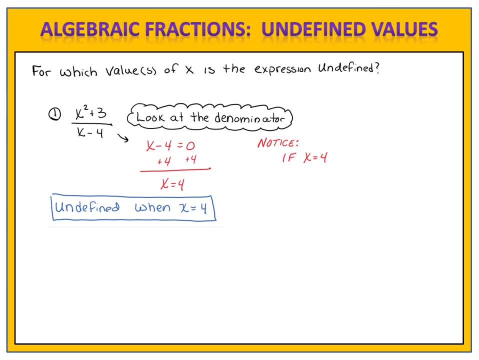 this: If x equals 4, here's what we have. In the numerator x squared plus 3 is 4 squared plus 3.. In the denominator 4 minus 4.. That would give us in the numerator 19, and in: 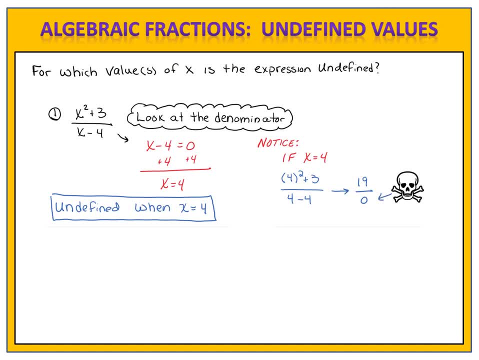 the denominator 0. We cannot divide by 0. It is undefined. Therefore x cannot be 4. for this algebraic fraction It is said to be the undefined value. Sometimes mathematicians will write this using set notation. They'll put the undefined values in these squiggly. 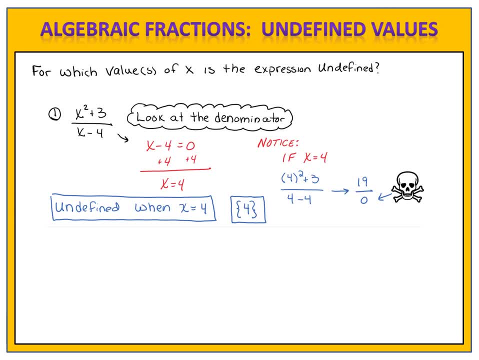 brackets, also called braces. in order to list them out, Let's look at another example here, This one for you to try. â We have an algebraic fraction: x squared minus 1, divided by x plus 8. Can you identify the values that make this expression undefined? Please pause the video here and 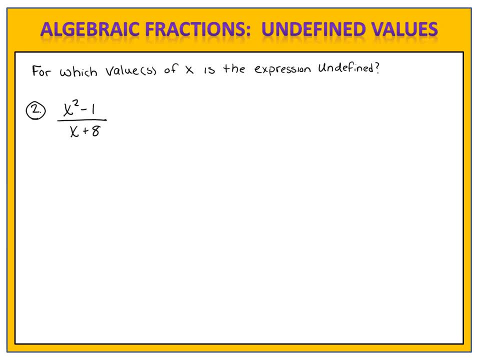 give it a try. Let's compare answers. We want to know what values of x cause the denominator to equal 0. So we look at the denominator x plus 8, and we make it equal to 0. We solve for x. 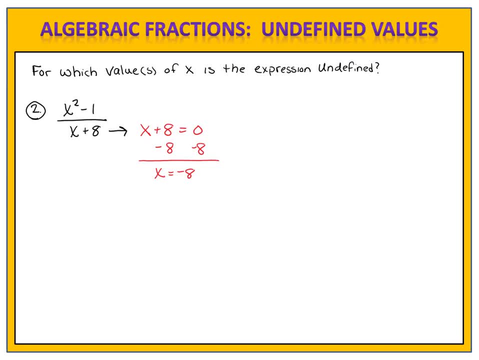 and we find that x equals 5.. equals negative 8.. This fraction is undefined when x equals negative 8.. We could also choose to write this using set notation, putting the negative 8 in the squiggly braces. Remember why negative 8 is the value that makes this fraction undefined. If we were to substitute: 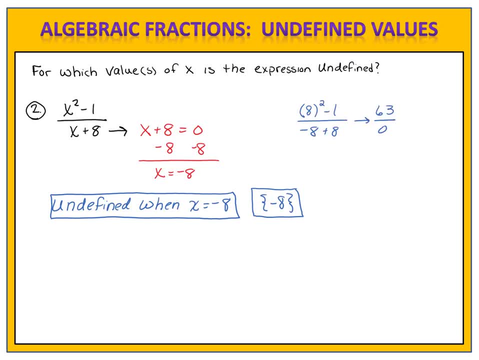 negative 8 in place of x, we would find that we have 63 divided by 0.. We can't divide by 0, and therefore negative 8 is an excluded value. It causes the fraction to be undefined. Here's another one for you to try. Can you find the values of x for which this expression? 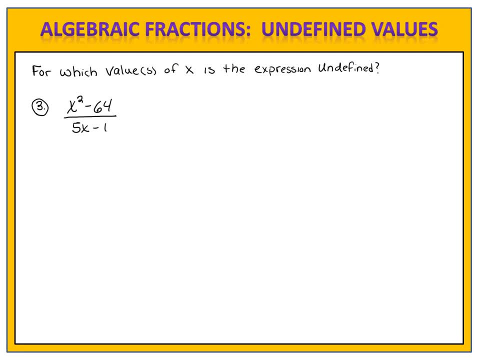 is undefined. Please pause the video here and come back when you're ready to compare answers. Let's compare answers. We want to know what values of x would cause the denominator to equal 0. We set the denominator equal to 0 and then we solve the resulting equation. We go through a few steps to get there and 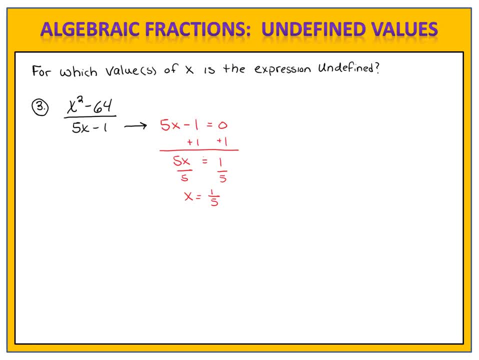 we find out that x equals 1 fifth. 1 fifth is the excluded value that causes the expression to be undefined. So this fraction is undefined when x equals 1 fifth. We could, of course, choose to write our answer in set notation. Sometimes these problems can be a little bit. 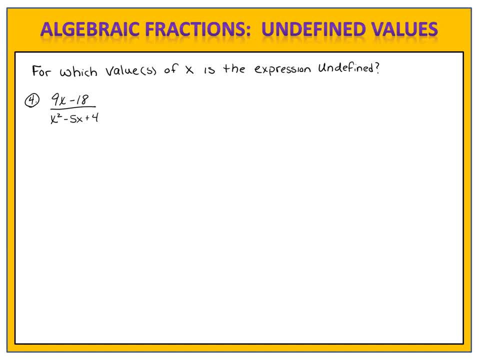 trickier. Look at example 4.. Here in the denominator we have a trinomial, and it's much more difficult to solve this equation because we have both an x squared and an x. So here's how we'll do it: We will factor the denominator and then set each of the factors equal to 0.. Here's: 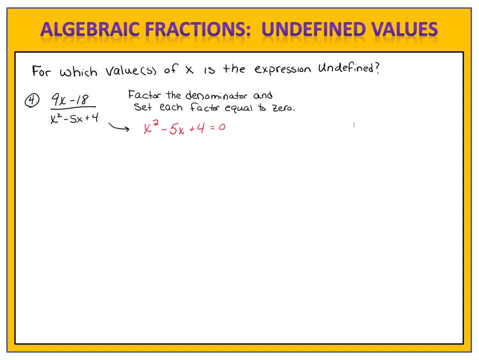 how it's done. We want to look at the denominator x squared minus 5x plus 4, and then we'll set it equal to 0.. In order to solve this equation, what we have to do is we have to begin by factoring. We factor the polynomial to x minus 1 times x minus 4.. Then we look. 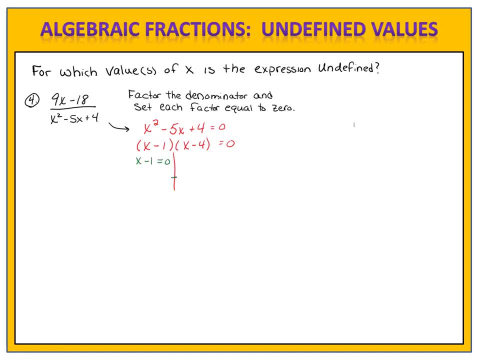 at each factor separately. We look at the x minus 1 and set it equal to 0, and we look at the x minus 4 and set that equal to 0. We solve each of those little equations. On the left, we have x equals 1.. On the right, we have x squared minus 5x plus 4.. On the 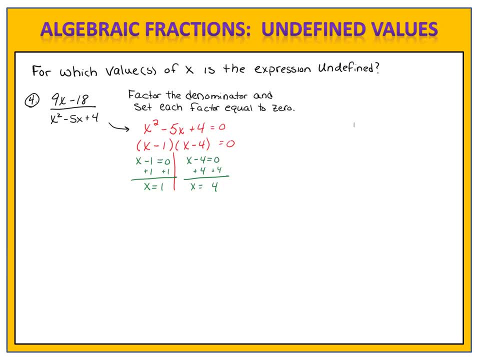 right, we have x equals 4.. Those are the undefined values. This fraction is undefined when x equals 1 or x equals 4.. We could choose to list this using set notation. If you do, you separate the two numbers by a comma, Notice that I put the smaller number first and the 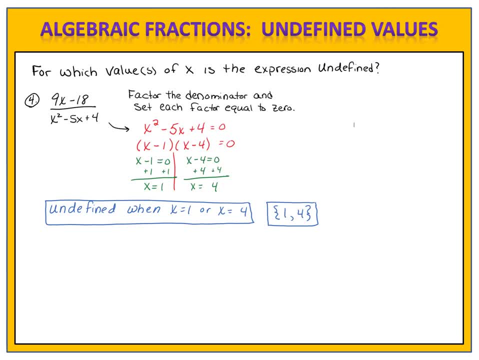 larger number. second, That's customary to do. Remember what these two values mean. They cause the original fraction to be 0.. If I look at the original problem, 9x minus 18 over x squared minus 5x plus 4, and for 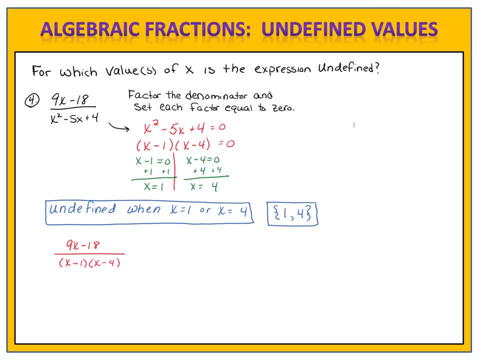 the sake of making life simple, I put the equivalent factored form in the denominator and I substitute those numbers, 1 and then 4, in notice what happens? I end up in the first case with a 0 in the denominator, Negative 9.. 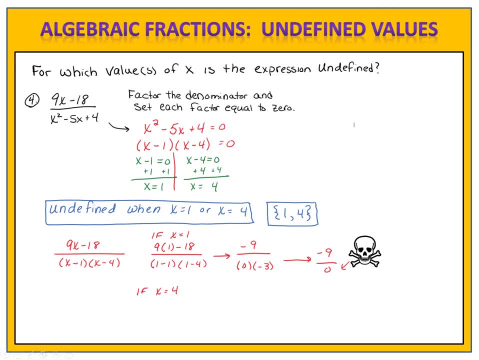 I end up with 18 over 0, and I know that that's not allowed. If x is 4,, something similar happens. I end up with 18 over 0. Again, there's danger in the denominator. We can never divide. 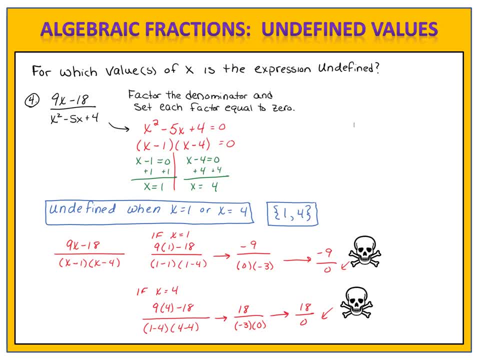 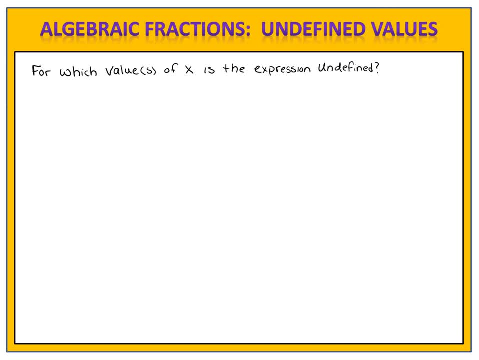 by 0.. Therefore, the excluded values are 1 and 4.. Here's one like that for you to try. For which value or values of x is the expression undefined? 9x minus 36.. 3 divided by x squared plus 7x minus 18.. Here we have a trinomial in the denominator. 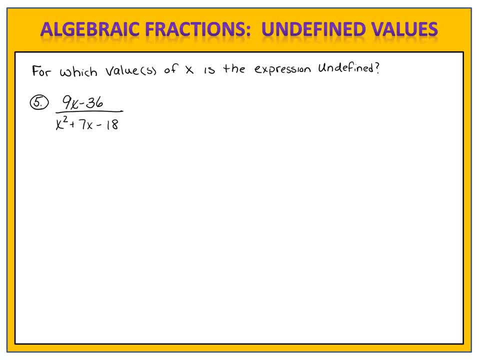 so we'll have to use our factoring trick, like we did in the last exercise. Please pause the video here. give this problem a try and come back when you're ready to compare answers. Let's compare answers. We began by factoring the trinomial x minus 2 times x plus 9.. We then set each of those factors equal to 1.. As I mentioned in the first class, x is equal to 7x over 0. In this case, if x is 0, then I milk out this one. If x is 1,, then I milk. 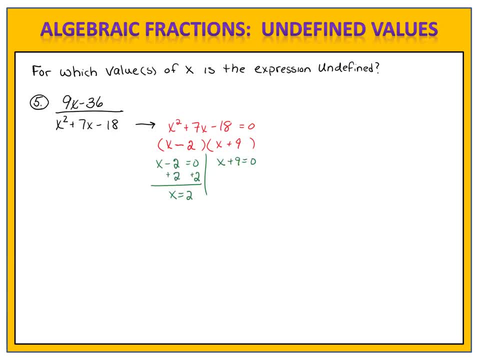 equal to 0, and solve each one separately. x equals 2 and x equals negative 9.. These are the two values where the fraction is undefined. so the fraction is undefined when x equals 2 or x equals negative 9.. Remember, you can write this using set notation. be sure to 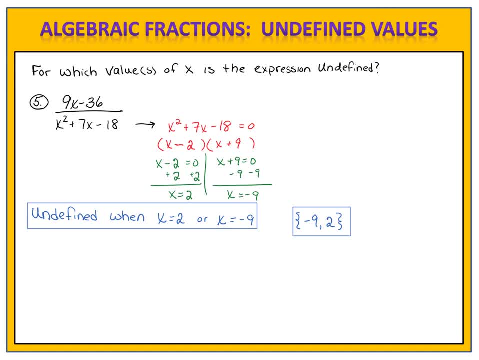 put the smaller number first and the larger number second. Let's end with one last example for today: x plus 8 divided by x squared minus 49.. You might recognize that denominator as a difference of two perfect squares which can be factored. 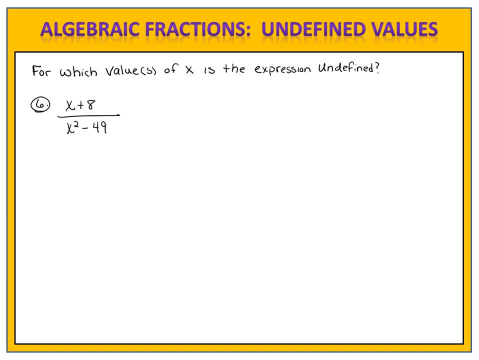 Go ahead and find the undefined values for this fraction. Please pause the video here and come back when you're ready to compare answers. Let's compare answers. We begin by looking at the denominator x squared minus 49 and setting it equal to 0.. 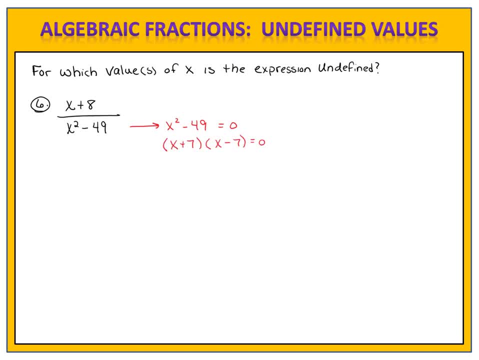 We then factor x plus 7 times x minus 7 equals 0.. We look at each factor separately and set that factor equal to 0. When we do, we find that our excluded values are negative 7 and positive 7, so this fraction is undefined when x equals 7 or negative 7.. If you choose. 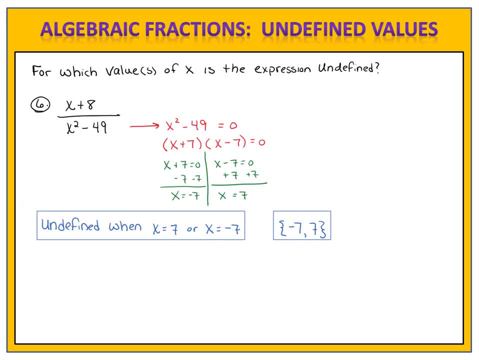 to use the set notation. be sure to put your smaller number first and your larger number second. Something really cool happens here. Notice that we have both positive and negative 7 at the same time. We can actually consolidate that into a single statement We can write. 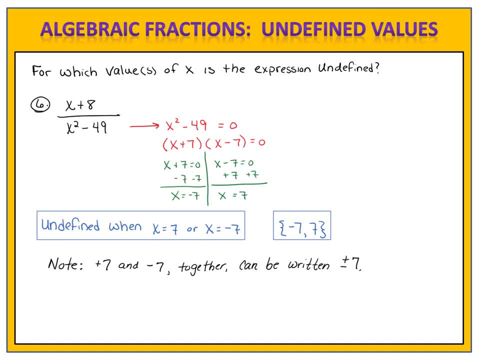 positive and negative 7 together as plus or minus 7, with a little plus or minus symbol, which denotes positive 7 and negative 7.. And if you choose to do that, you could say that this is undefined when x equals plus or minus 7, which means that x is undefined If you. 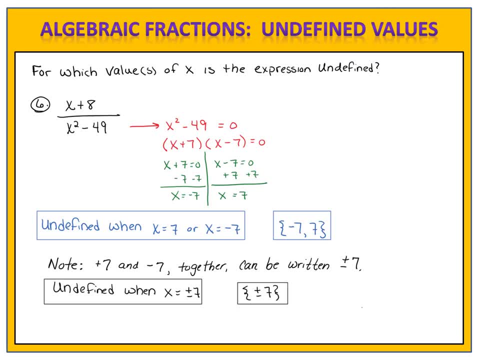 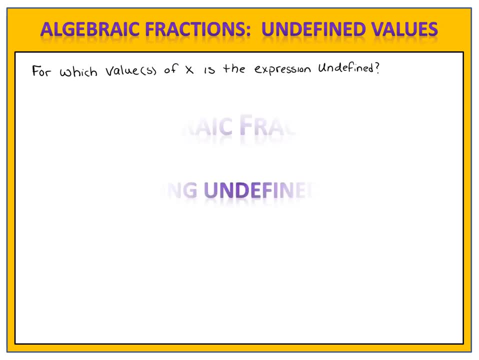 choose to use the set notation. you can write positive 7 and negative 7 as well as using set notation, And that's everything you need to know to get started working with algebraic fractions. You now know how to identify undefined values and you're ready to go.